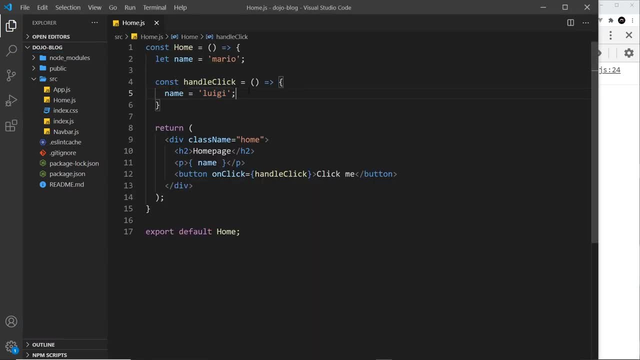 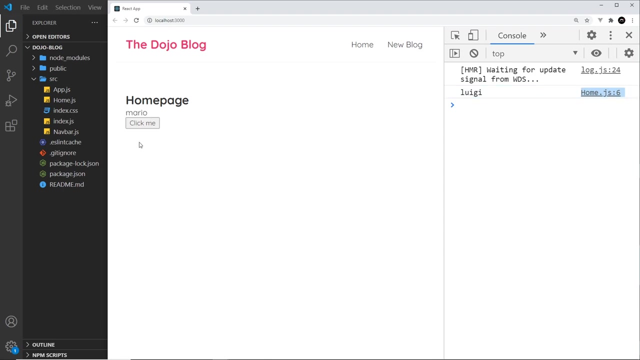 It doesn't change in the template. Now. the name itself changes and I can demo that by logging it to the console. So this value right here that changes. So if we see this, click me. we see, Luigi. It just doesn't update in the template. Now it doesn't update in the template because 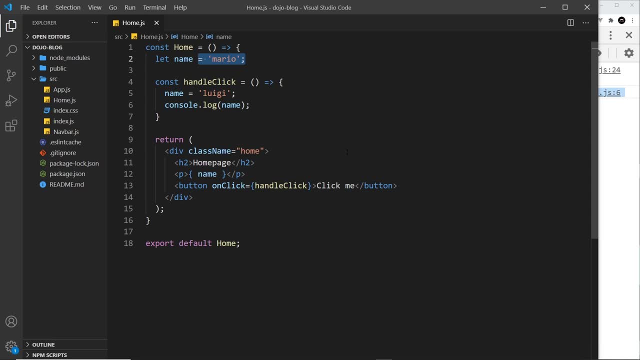 the variable that we created over here is not reactive Now. by that I mean that react doesn't watch it for changes or react to it. So when the value does change, it doesn't trigger react to re-render the template with that new value inside it. Nothing happens and we continue to see the old value in the browser. So in order. 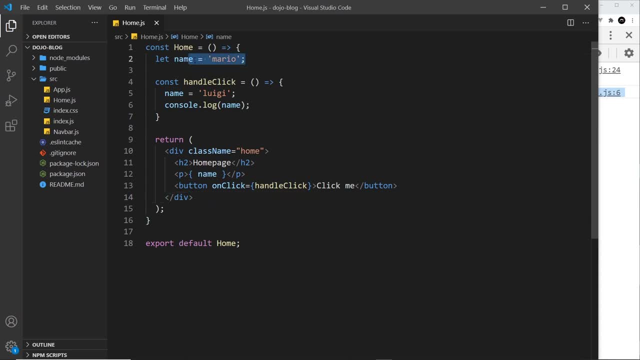 for this to work, we have to make the value reactive so that when it changes, react detects that and it re-renders the template where we output that value and we see the new value in the browser. Now, to do this in react we use something called a hook and that hook is: 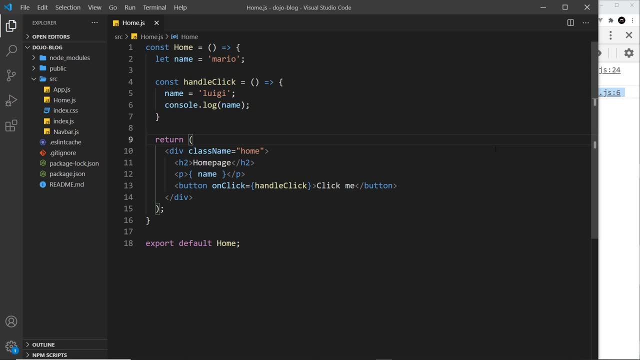 called use state. So hooking react is a special type of function that does a certain job and you can tell a hook by its name because it starts with the word use. So the use state hook gives us a way to make a reactive value and also provides us with a way to change that value whenever we 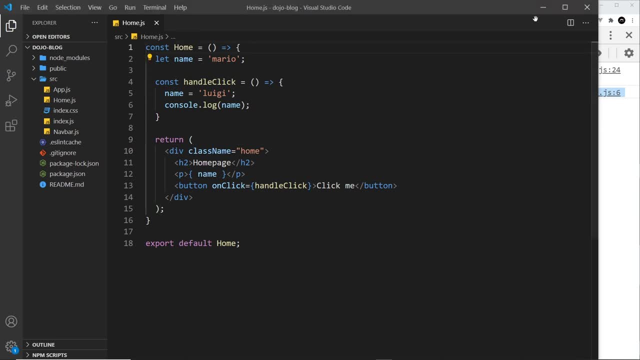 want. So in order to use this use state hook, first of all we need to import at the top of the file. So we say import, then curly braces, because we're going to destructure the use state hook and that is from the react library. So this grabs us the function from the react. 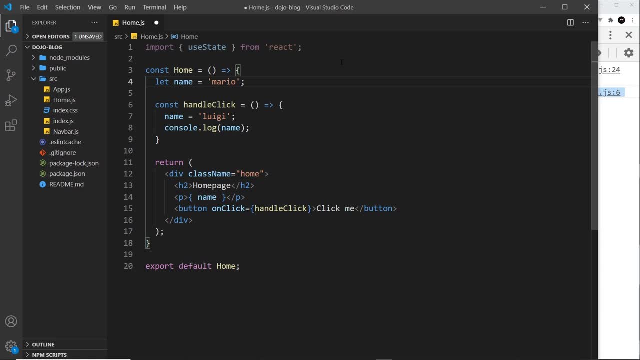 library and now we can use it inside our component. So let me just comment out this stuff right here and also delete this inside handle click, and instead we're going to make a reactive value using use state, and the way we do this is by saying use state, which is a function, so we invoke 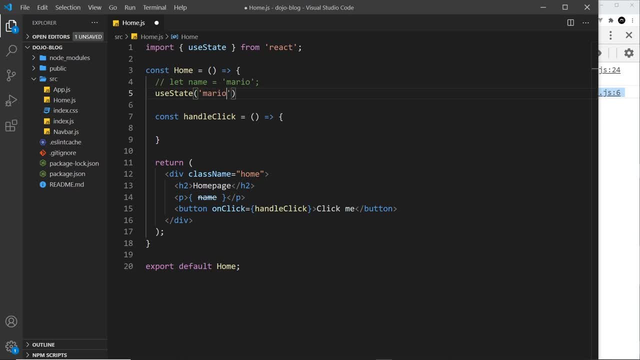 it and we give this state an initial value. So, for example, Mario, Now we want to store this in some value, because at the minute we're not storing it, we're just invoking the function. so the way we do that is by saying const, and then we use array destructuring to grab two values that this hook. 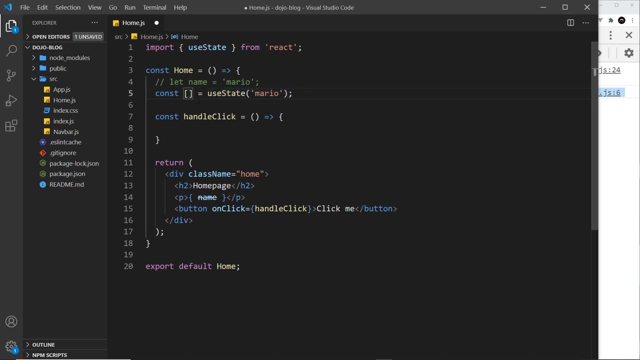 returns to us. So, first of all, the first value is this initial value, so we can call it what we want. I'm going to call it name. and the second value is a function which we can use to change that value, and most of the time you're going to see this called set, and then whatever we call, 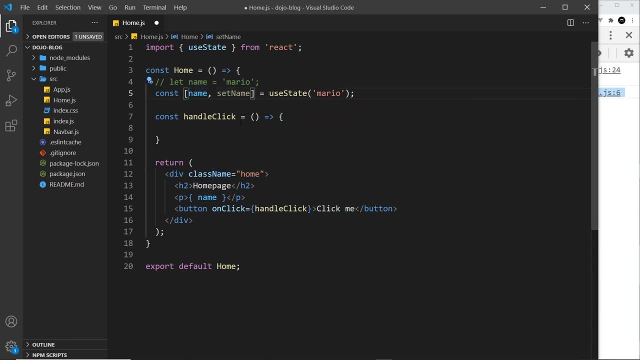 the value, so in my case, name. So now, if I was to use this value in the template, it's going to get us whatever the value of that state is. So, Mario, to begin with, and then if we want to change that value, we can use this function to do it. So I could say down here, set name and pass in a new. 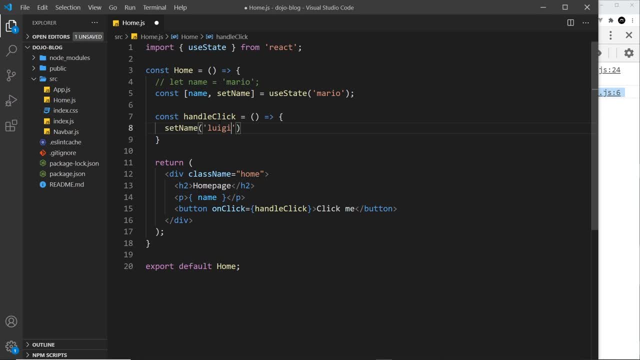 value, so I could change that to Luigi. and this value is reactive, this state value, so if it changes at any point it's going to change in the template as well. so when we use this function to change the value, that triggers react to re-render the component, and when it re-renders we have that. 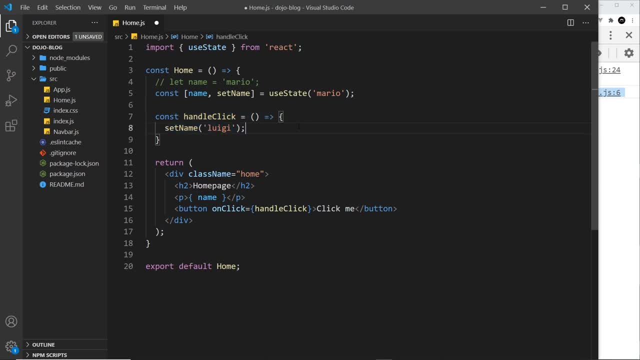 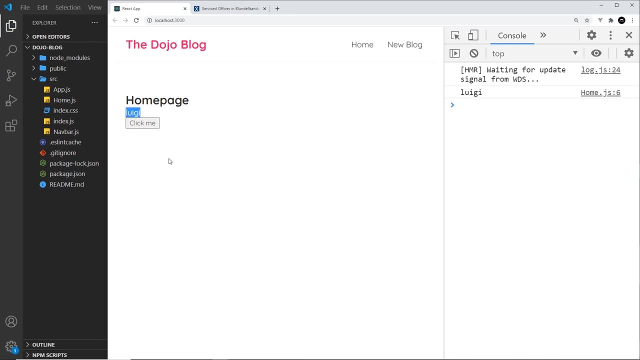 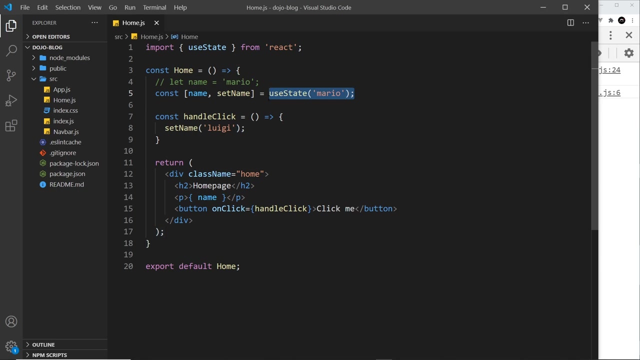 new value of name because it's been updated, all right, so let me test this out. I'm going to save it and come over to the browser and now, if we click on this, we see it changes to Luigi. awesome, so now this is reactive. This hook as many times as we want in a component for different values, and this value can be anything. 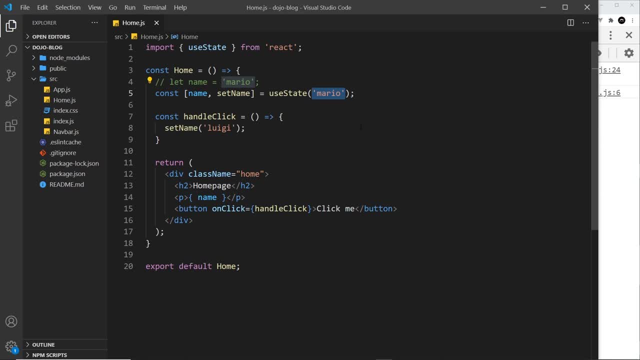 it can be an array, it can be an object, it can be a boolean or it could be a number. it really doesn't matter what the data type of the state is that we're using. so let's do another example, which is going to be a number. I'm going to call this age, so I'll use array destructuring to say: 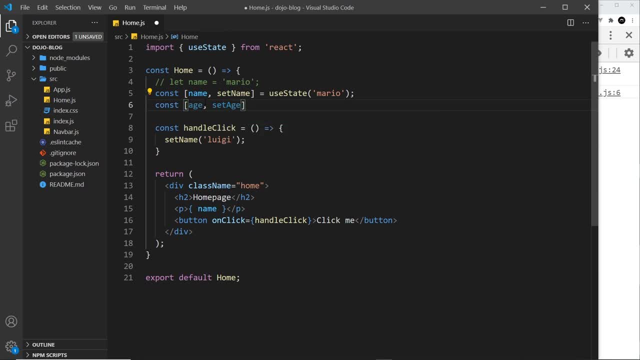 the value is called age and the function I'll call set age and we'll set it equal to use eight again. and we give this an initial value which I'm going to set to be 25, right, and now I can output that I'm going to say name is and then output the age and then I'll put years old.